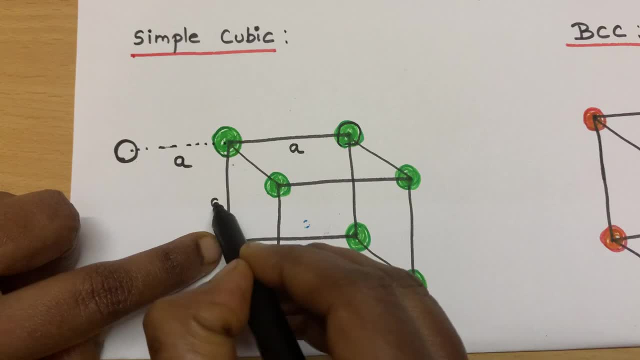 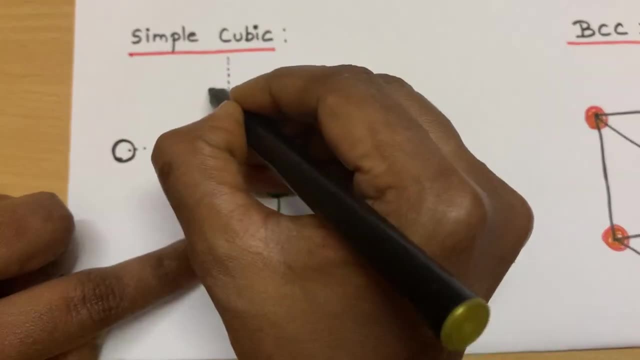 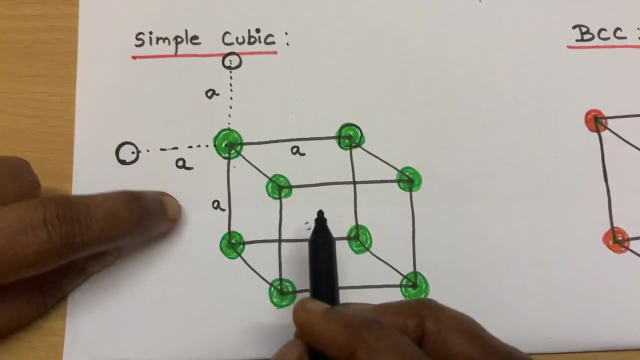 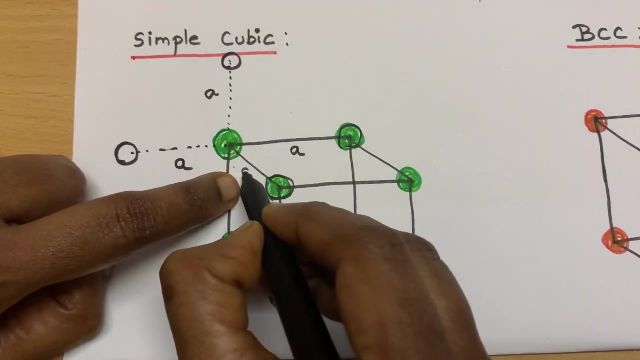 see there is one more neighboring atom downwards at an edge length of a. Similarly, there will be, and there must be, an atom at the same distance above also in the another unit cell. Okay, so here in the front side, in the front side, There is a neighboring atom near atom, which is present at a edge length of a, Similarly an atom. 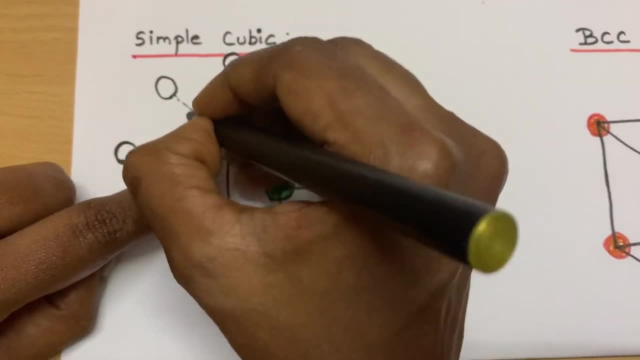 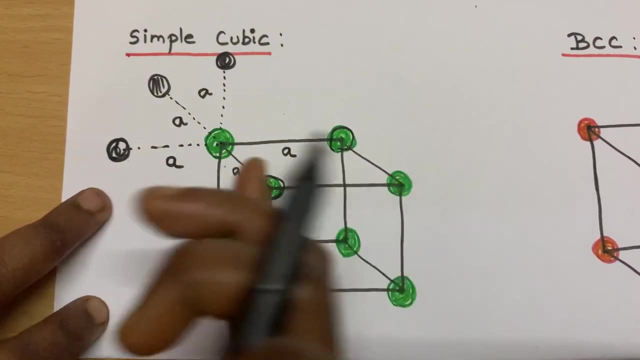 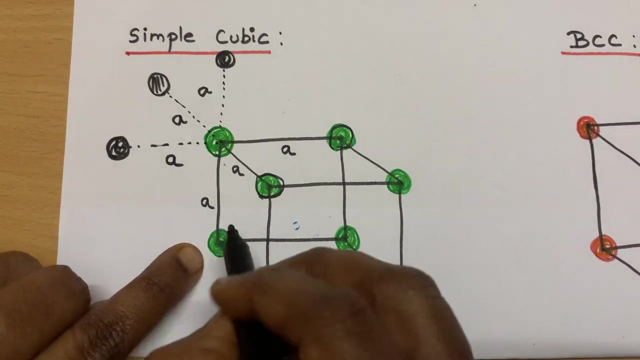 must be present at the backwards also, at an edge length of a. You got my point, students. You got my point. So right hand side, there is an atom. So similarly, at the same edge length, there must be an atom in the left hand side also. So bottom there is one atom, So above also there must be one. 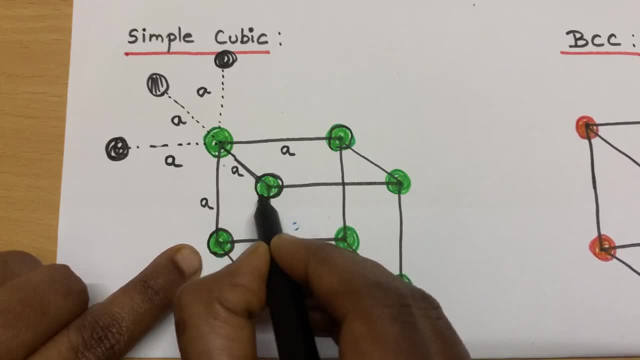 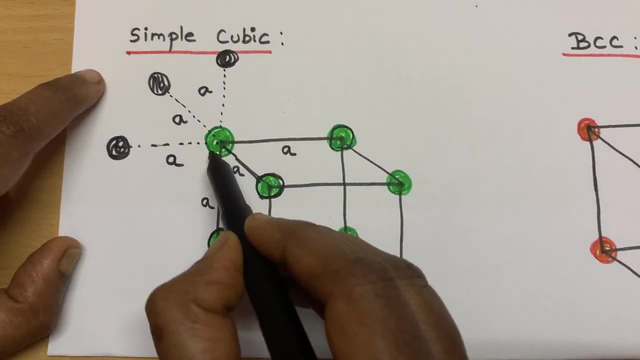 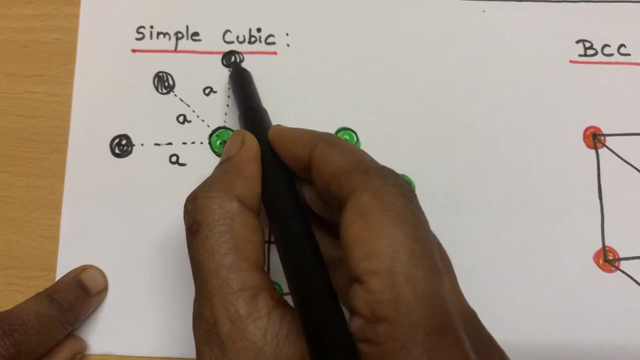 atom. So this is what Front side- Front side- there is one atom, So similarly back side also there must be another atom present. So totally, how many atoms are surrounding this particular atom? 1, 2,, 3,, 4,, 5,, 6.. 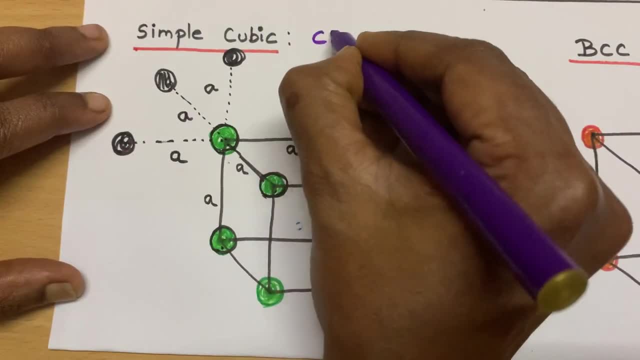 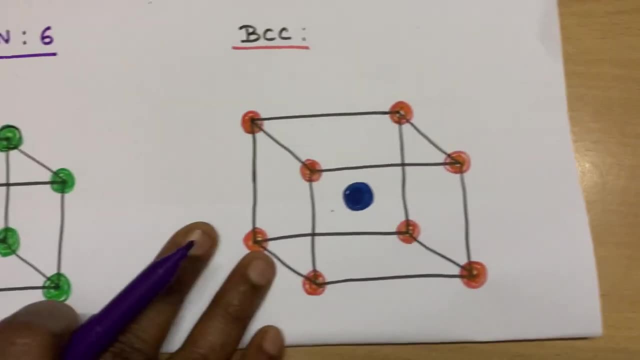 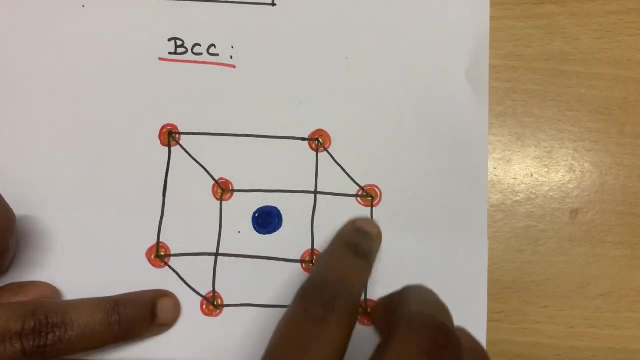 Okay, so the coordination number, So the coordination number of simple cubic system is 6.. Okay, got it Now coming to BCC. So in BCC, how the atoms are present, It is located at the corners. In addition to that, there is an. 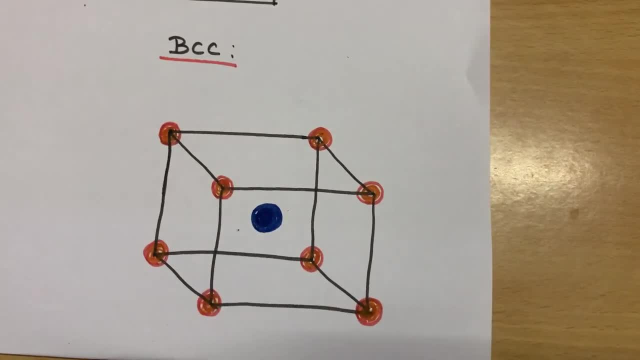 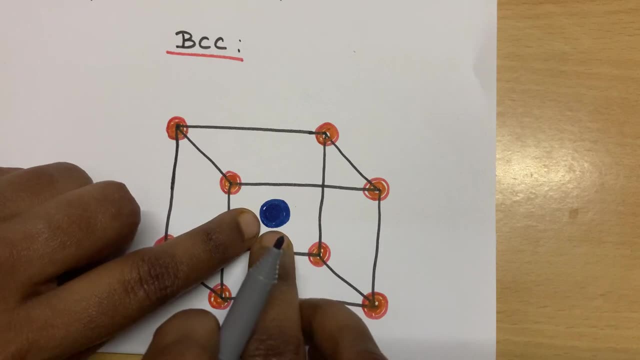 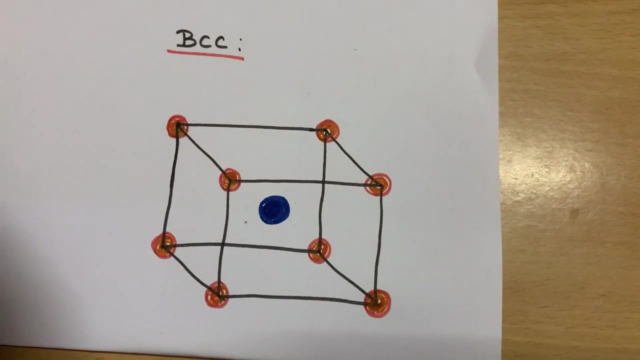 atom at the center, At the center right. So how to find it? You see, I am going to take this atom, One representative atom I am going to show. So we are going to take this. So we have to choose the nearest atoms. So you see how the body center cubic lattice is present. See, I have made a model. 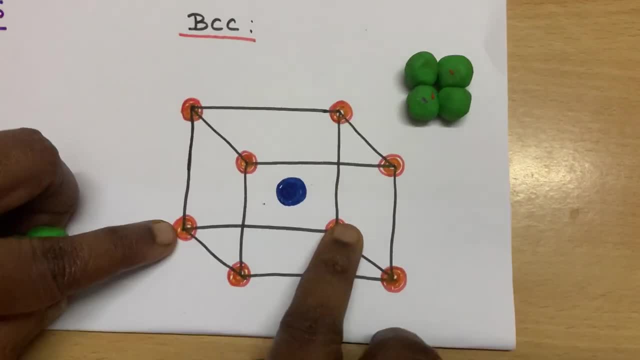 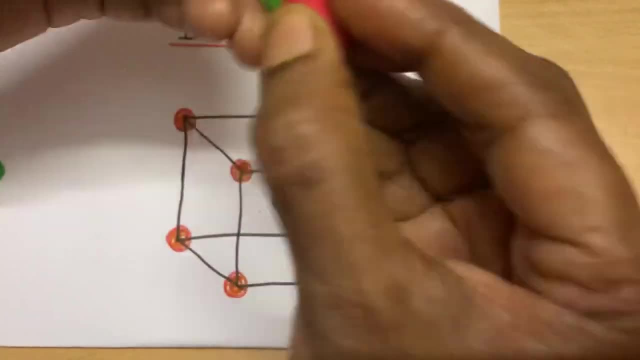 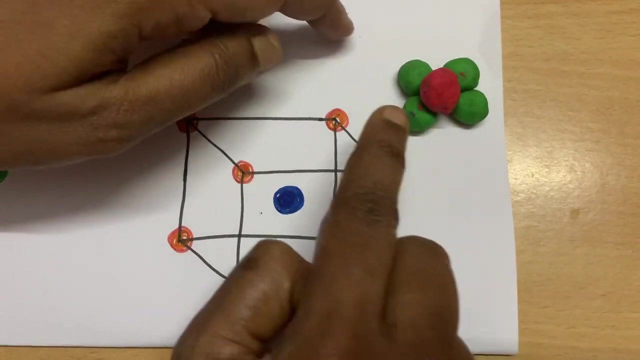 you see there are four atoms, okay, the one, two, three, four, four. they are not touching each other. they are not touching each other. okay, and there is an center atom, center atom. okay, center atom. you are placing it above, so this center atom is in contact with the bottom four. right, it is. 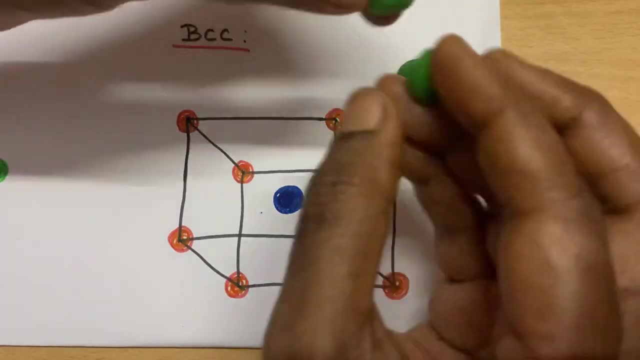 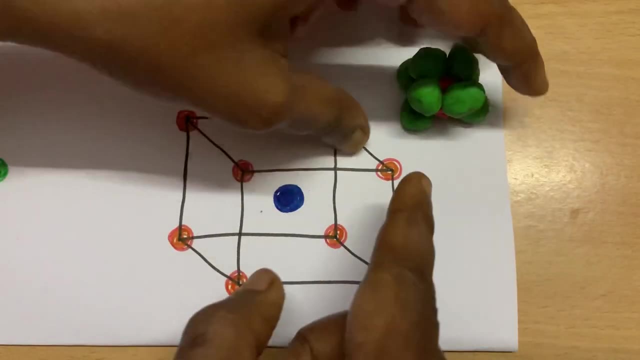 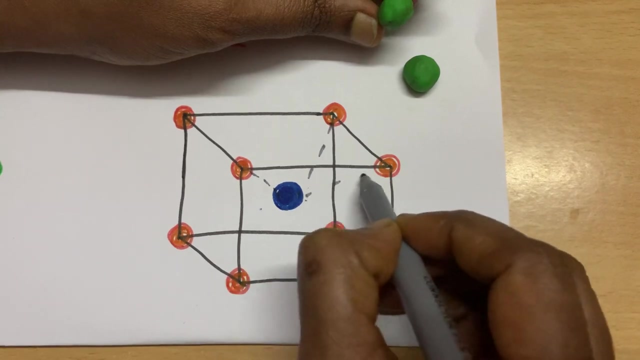 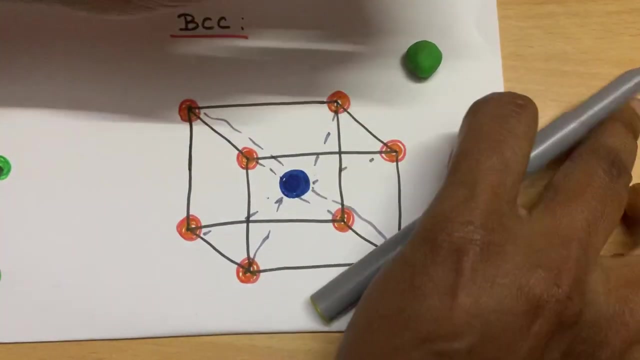 touching the bottom four- right, everybody agrees. and similarly it is touching a four more atoms above, also for the center atom. i am going to take the center atom, so this center atom is stitching. okay, the above, the above four atoms and the below four atoms. correct in this. 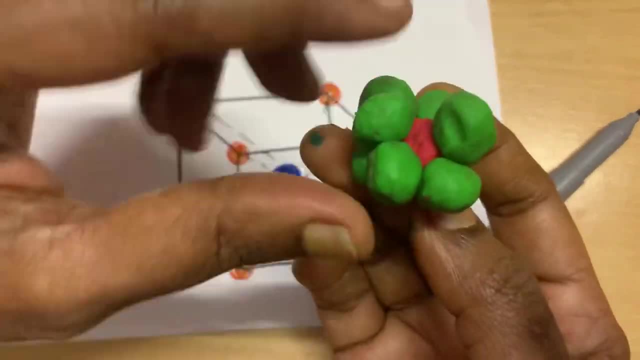 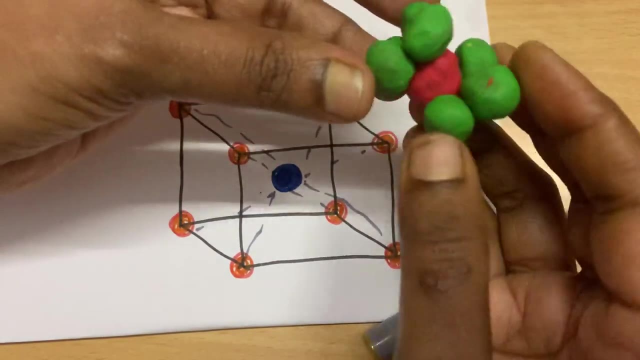 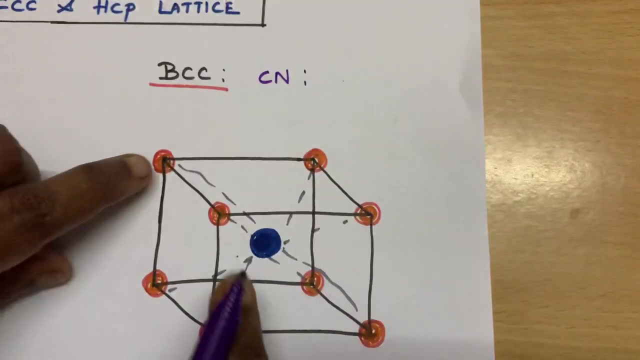 the center atom is stitching the above four atoms and the below four atoms. there are four atoms above and four atoms below. okay, so what is? the center atom is stitching the above four atoms and the below four atoms. there are four. the coordination number. so the coordination number for bcc is one, two, three, four, five, six, seven, eight. 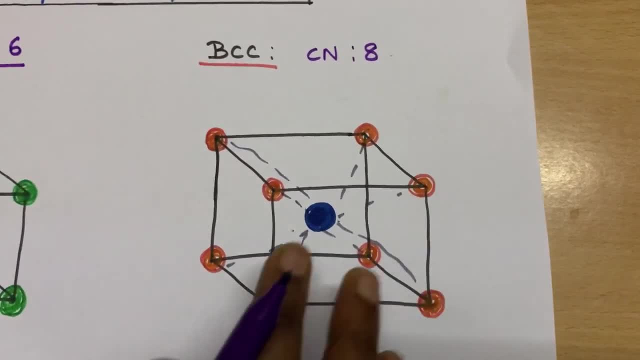 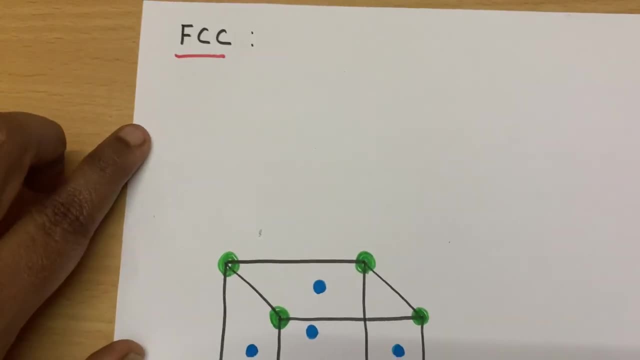 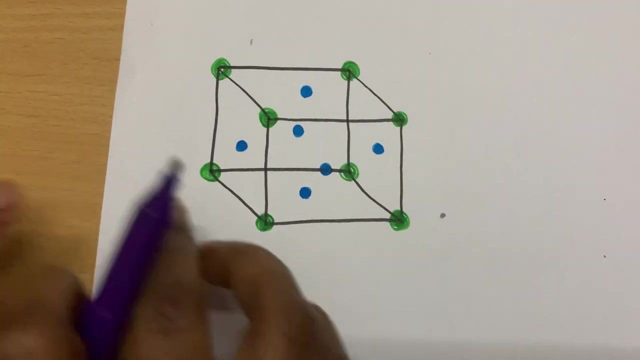 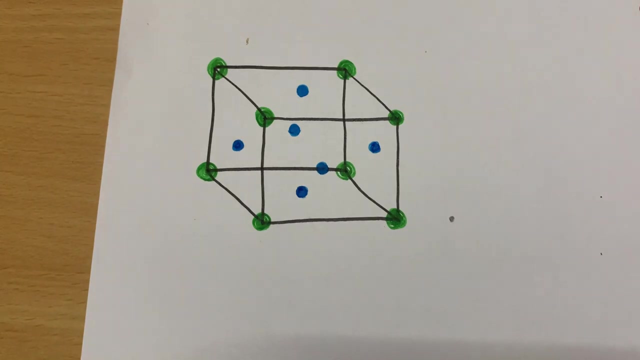 so eight. okay, for bcc, the coordination number is eight. so now coming to fcc. now coming to fcc. so we all know that in fcc the atoms are placed at the corners. in addition to that, it is also present in the face center. okay, so what i am going to take is: what is a representative atom? i am going to take is: 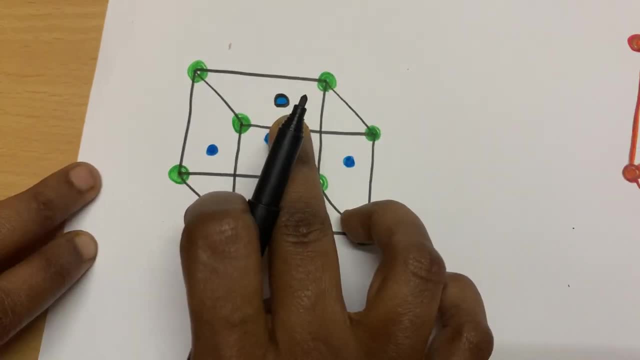 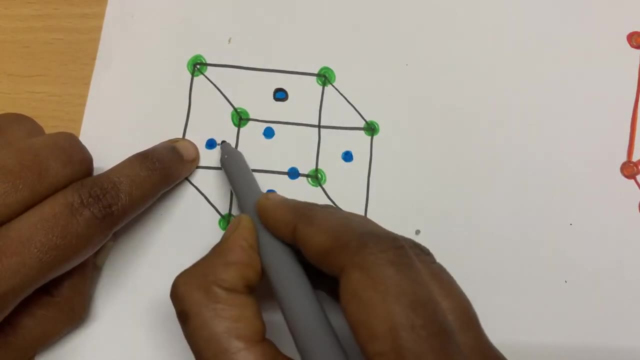 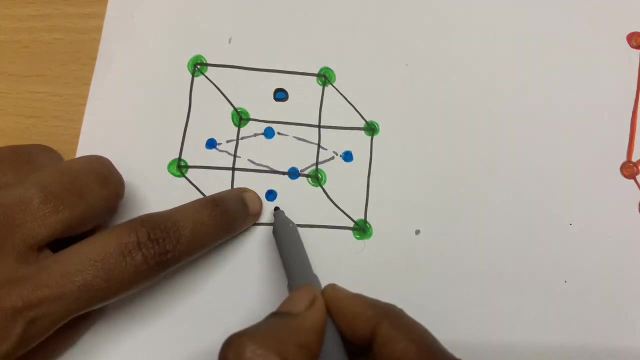 this atom i am going to take, so i am going to find how many atoms are connected to it. okay, so these four planes, you know, these four planes remind these four atoms remain in the same plane and this one below, and it is not connected to this because it is far away. 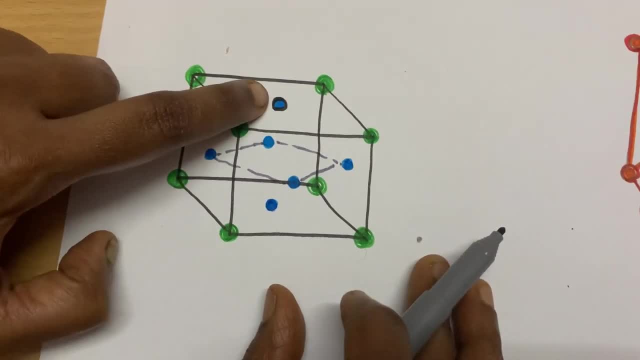 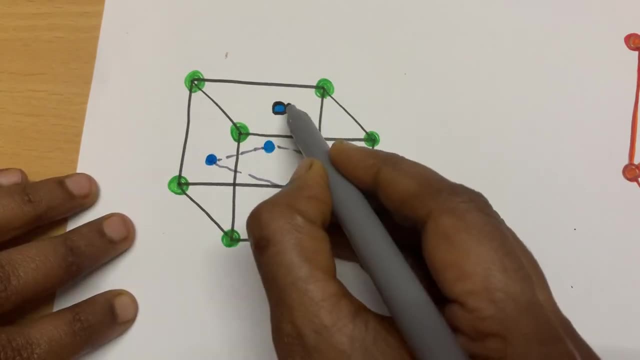 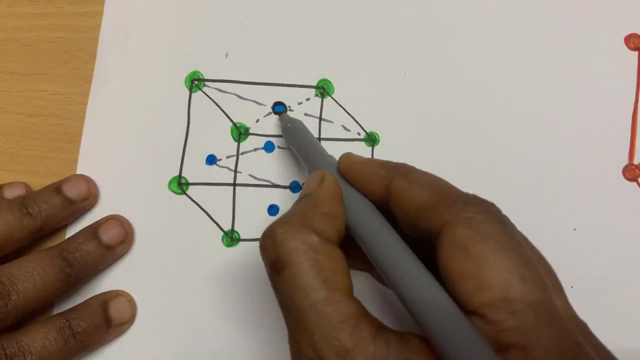 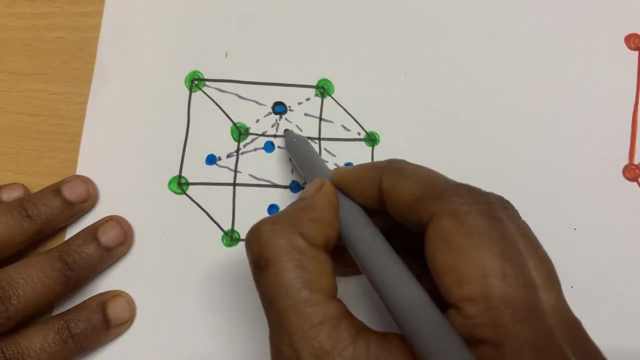 it is. i am going to check the coordination number for this atom and for that we have, i have to choose only the nearest atom, okay, so obviously this atom will be coordinated to this. okay, and it is coordinated to these four. okay, see, like this four there must be. there is an. 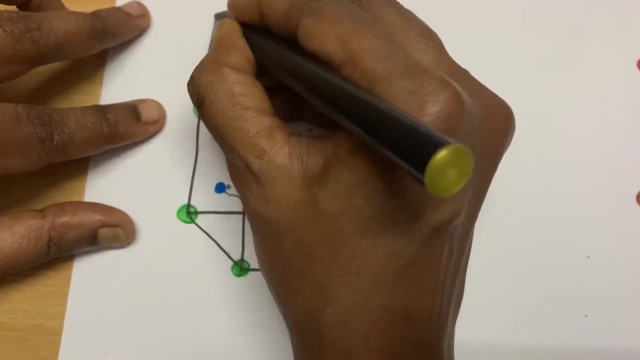 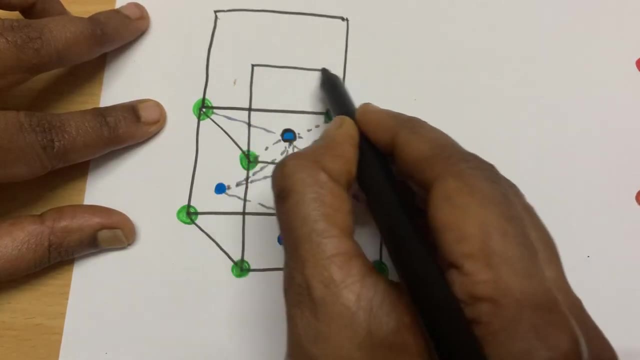 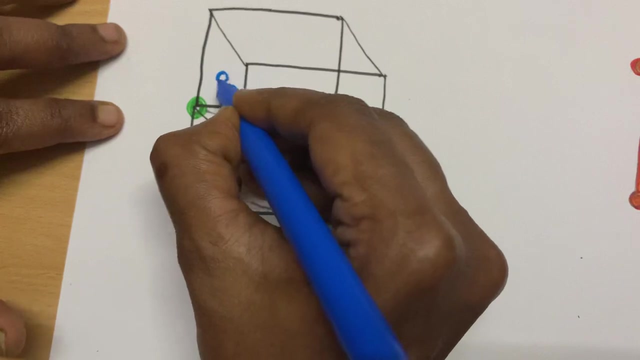 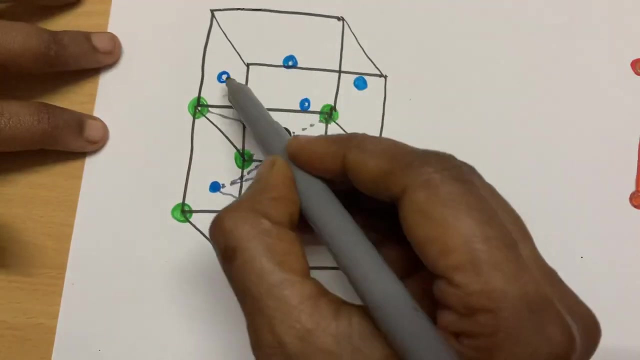 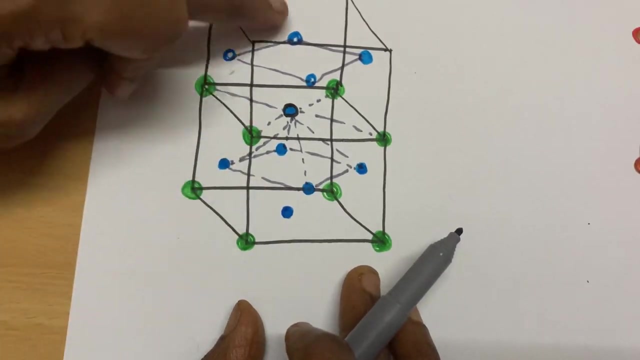 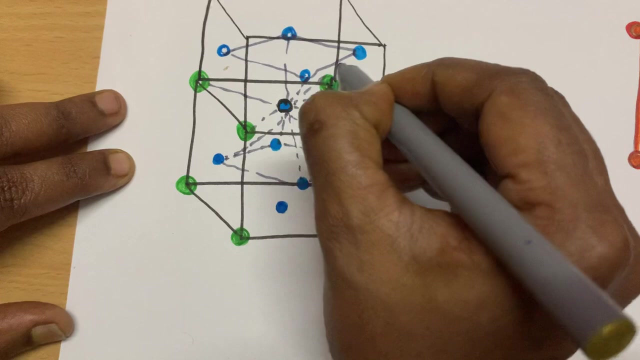 one another. one more unit cell above? no, so there must be. there is one more unit cell above, okay, and there will be. these four will be. similarly, it is below four atoms, above also will be four atoms, okay, so this atom will also be in contact with these four. 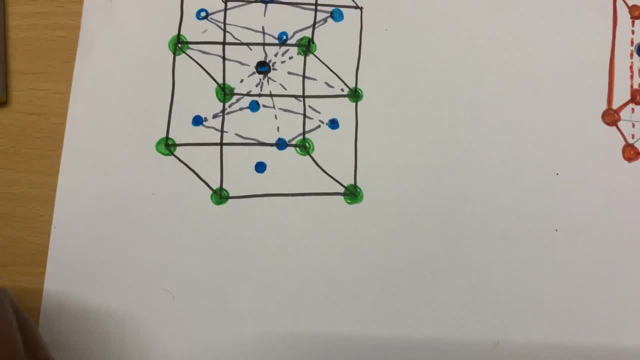 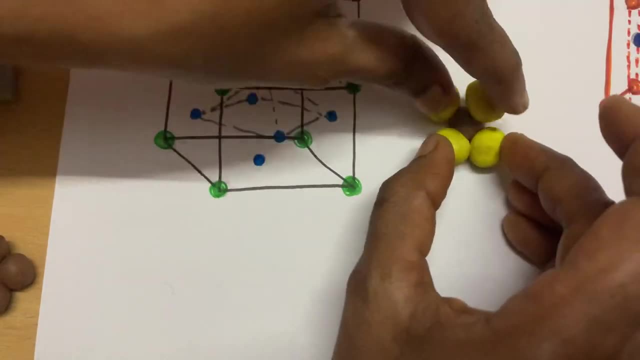 okay, I will show you. what is this. see, I am going to take this plane, okay. so what is that? this plane is this one, okay? 1,, 2,, 3,, 4, the center atom is this one? okay? so down there is. 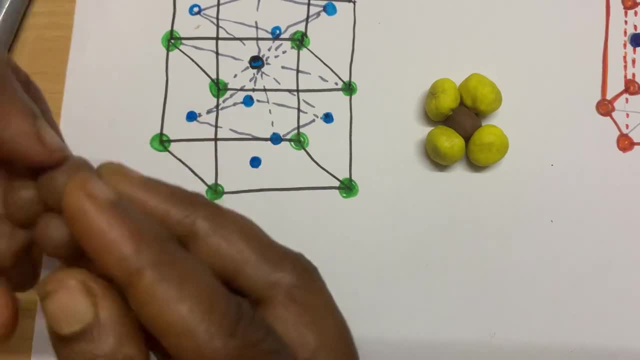 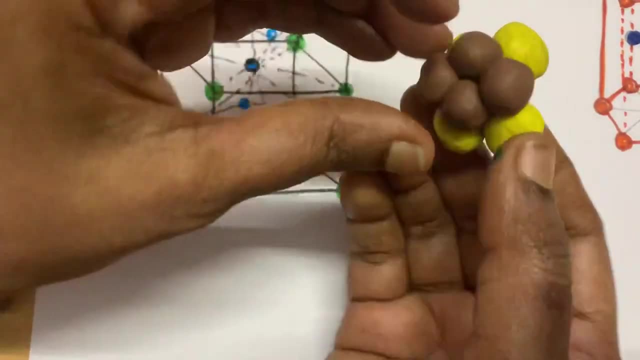 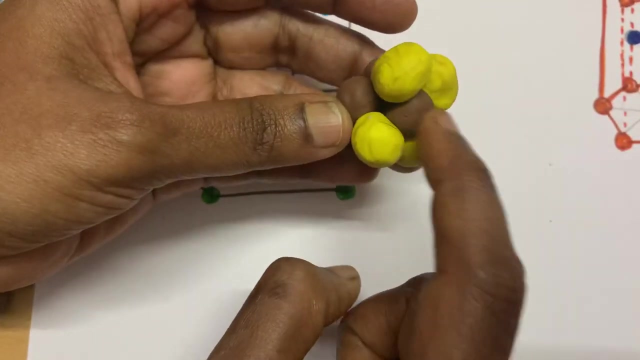 face centered atoms. how many face centered atoms? 1,, 2,, 3,, 4, so I am going to place it like this: this four, this center atom, now it is connected to these four, the four, this is corner atoms. I have given the yellow color and this is also face centered. all these are face. 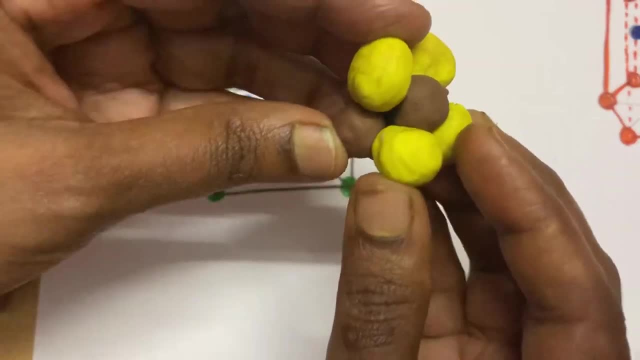 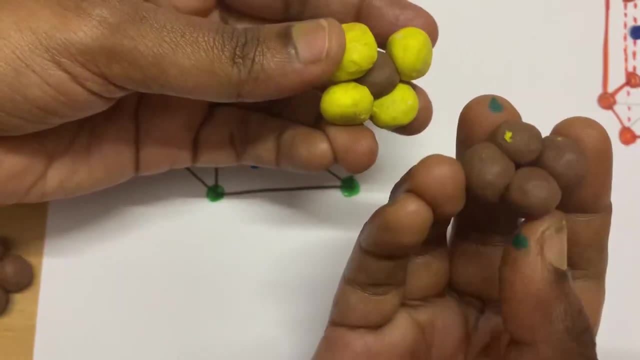 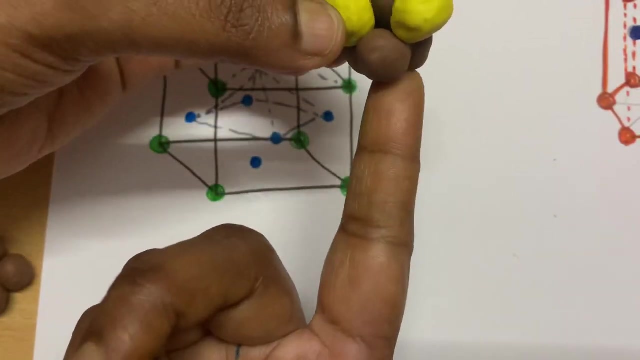 centered. all these are face centered. okay, so actually it will be like this: only so this center atom is in connected with this corner four atoms- and also with the, the four face centered atoms, and in the below there are four atoms. there must be above also. 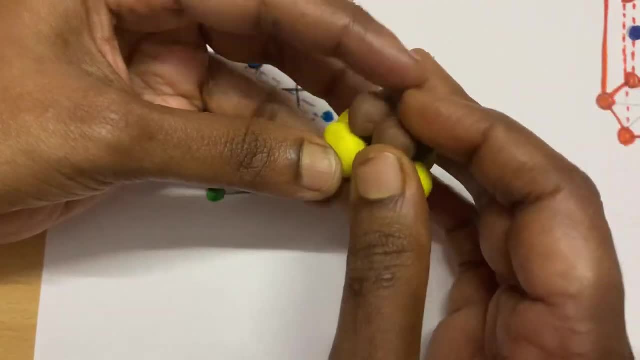 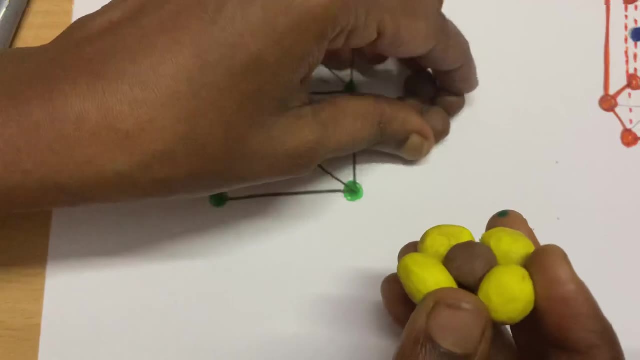 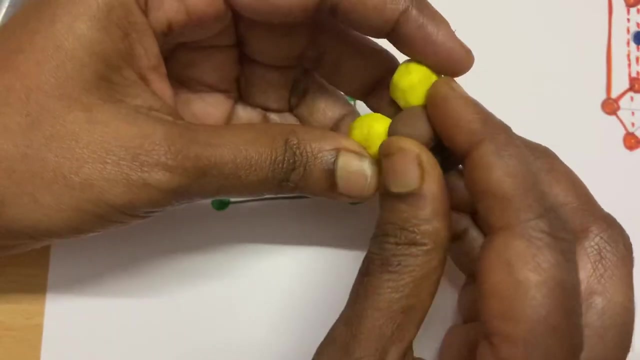 there must be four atoms, so I am going to place another four. so this particular center atom, it is in contact with what? 1, 2, 3,, 4,, 5, 6,, 7,, 8,, 9,, 10,, 11,, 12,, correct it is? 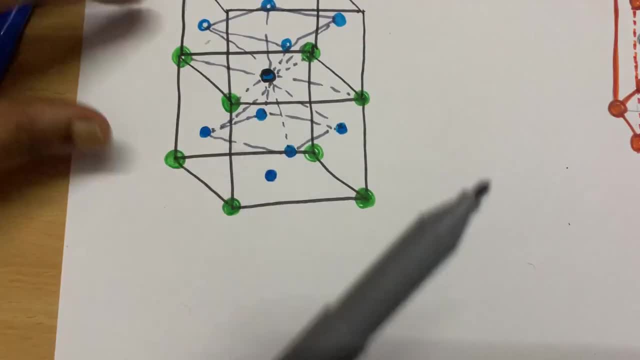 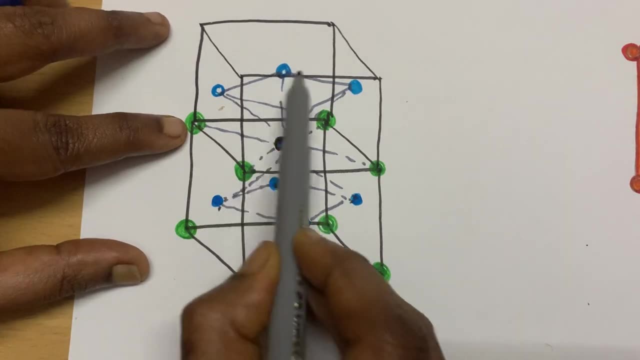 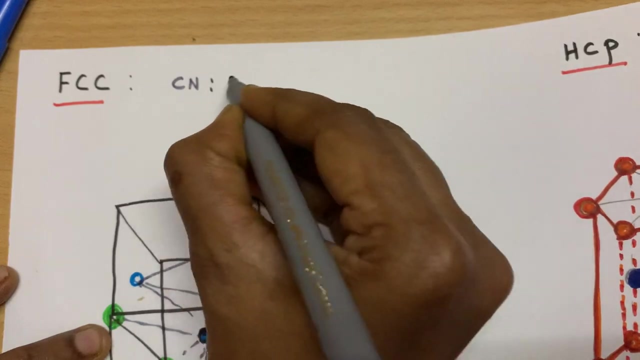 in touch with 12 atoms: 1,, 2,, 3,, 4,, 5,, 6,, 7,, 8,, 9,, 10,, 11,, 12, so the coordination number of the face centered cubic lattice is 12,. you understand, students, it cannot coordinate. 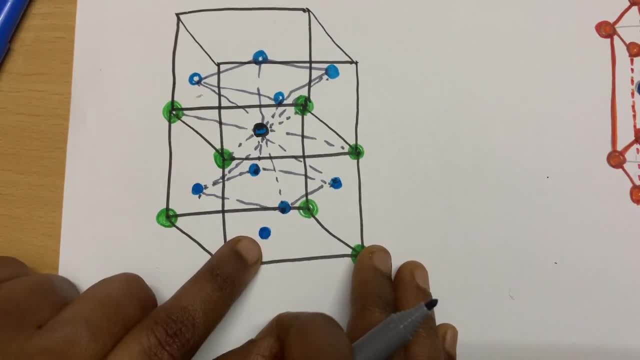 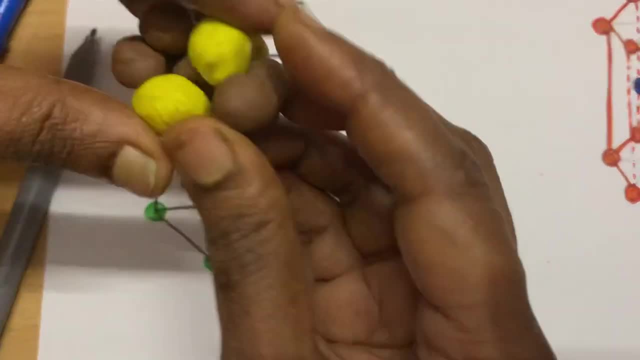 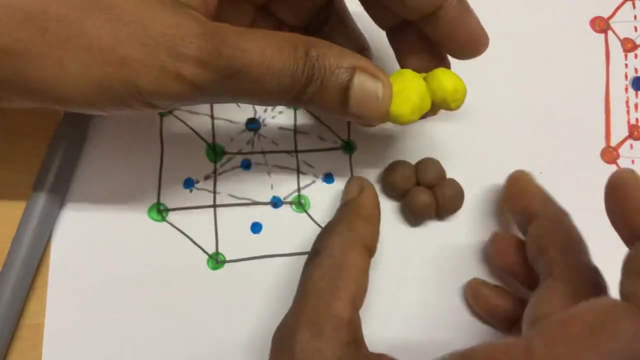 with this atom because it is far away. it can coordinate, it can be in touch with only the nearest atom. see, these remains in one plane, as I show you. I showed you, this remains in one plane and this five atoms remains in another plane. so okay, this pattern okay. 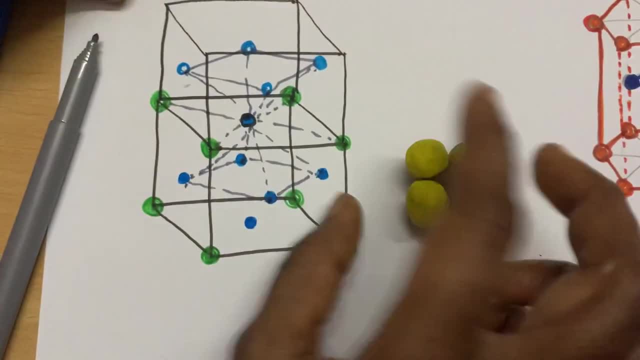 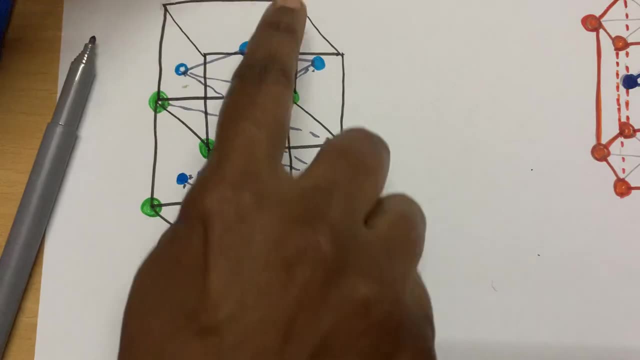 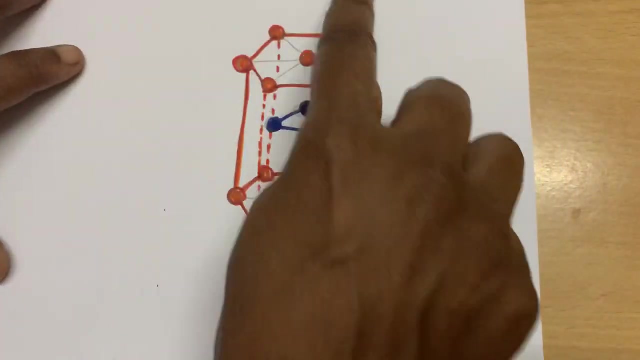 this another plane, okay, and this four atoms in the above plane. so okay, the center atom is in touch with coordination number. what four 12 atoms? so the coordination number is 12, so now coming to HCP. HCP is what you see: hexagonal close packing systems. so there, 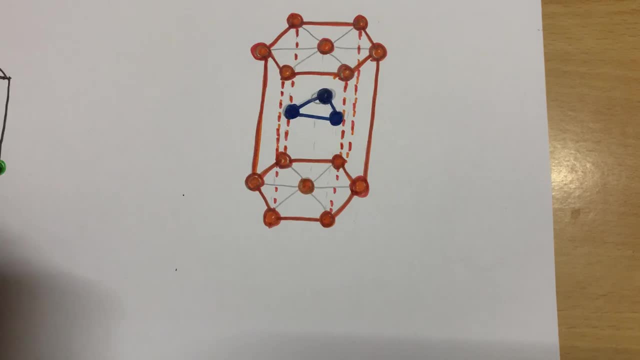 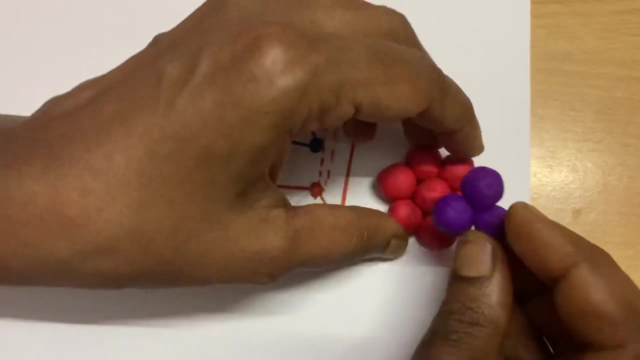 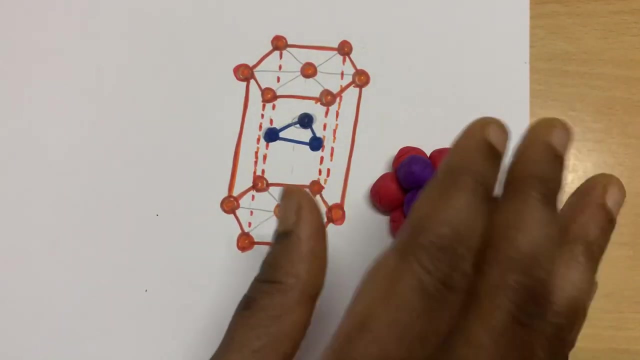 is. I will show you the model. okay, so it will be like this, repeating six atoms like this, and there will be some three atoms, three atoms like this, three atoms like this and above one more, six atoms. so like this it will be. it will be like: this is A, this is B, this is A. 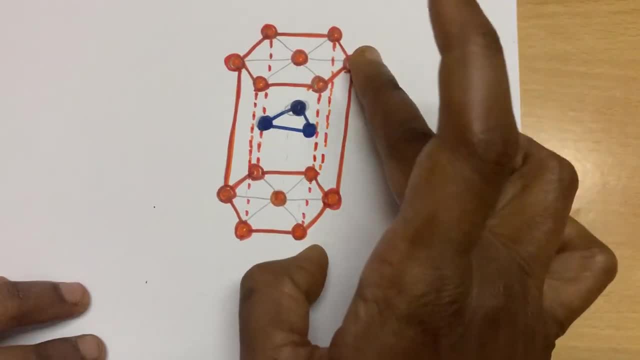 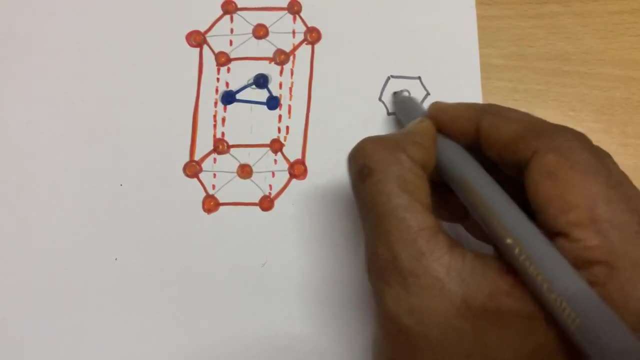 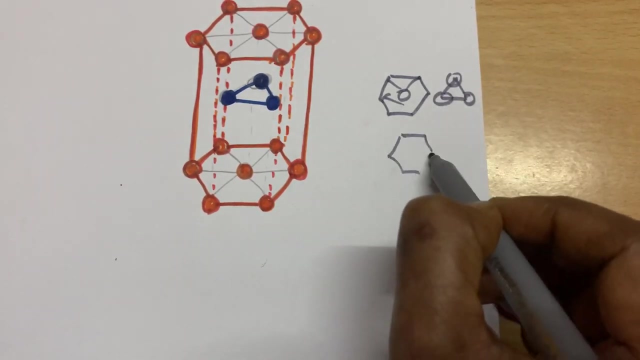 this is B, like that. so A, B, A comprises of one unit cell. okay, so one hexagon. okay, one hexagon center atom. one will be there. okay, above that there will be a triangle, three atoms, and again you have to repeat, and again you have to repeat. so A, B, A, like that. 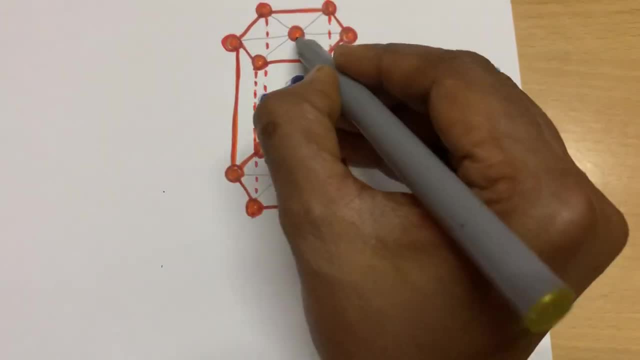 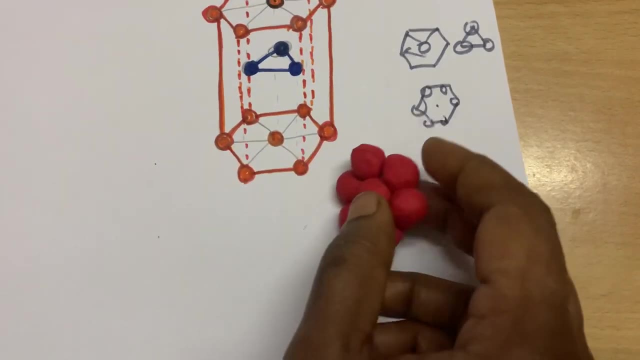 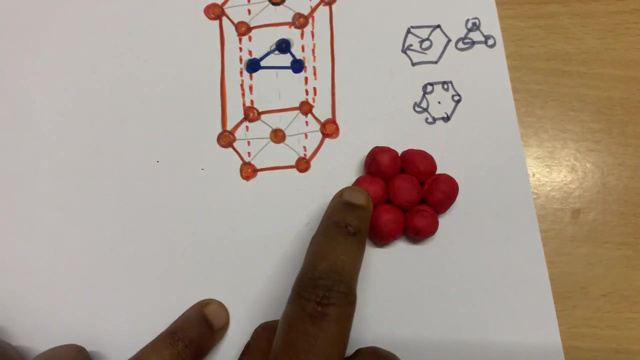 so what I am going to take is I am going to take this one as the representative atom and I am going to choose the coordination number, so I will tell you. so this one is the center atom, so it is coordinated with what? 1,, 2,, 3, 4,, 5, 6 already coordinated. now down there is a three atoms. okay, 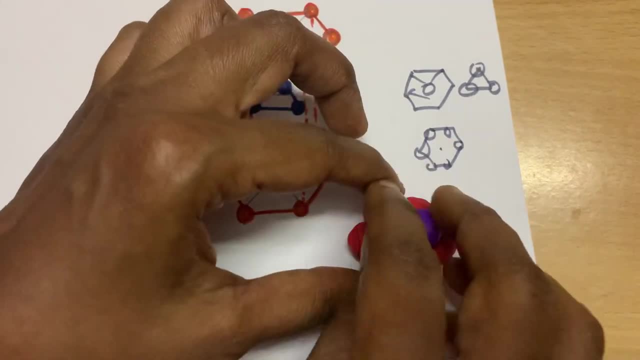 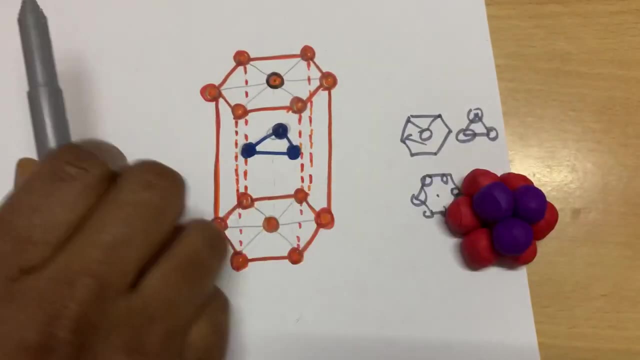 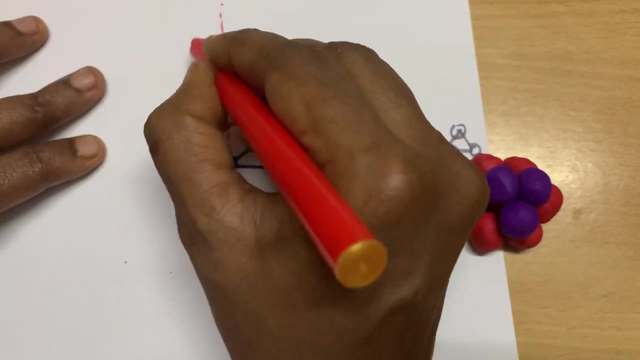 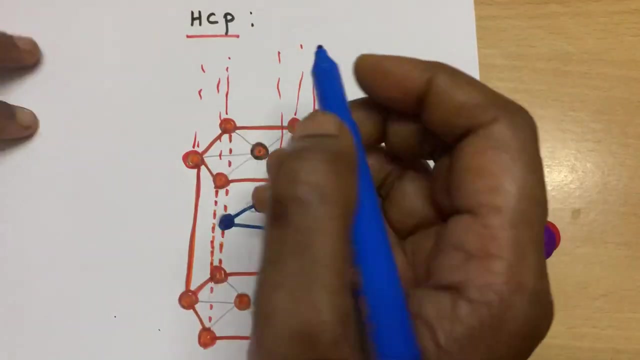 so the center atom is in touch with all the three atoms. center atom is in touch with all the three atoms. so like this: in the above unit cell there must be an. there must be a two unit cell above also. okay, okay, so there must be the three atoms above this. 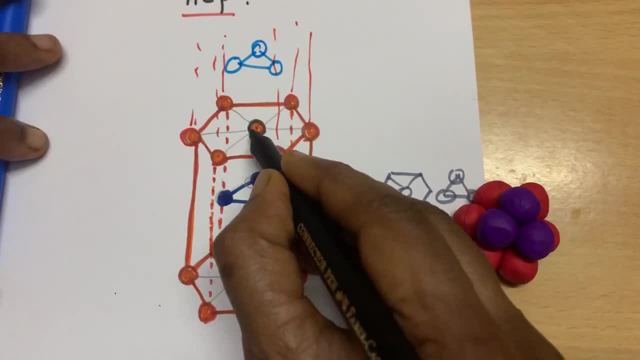 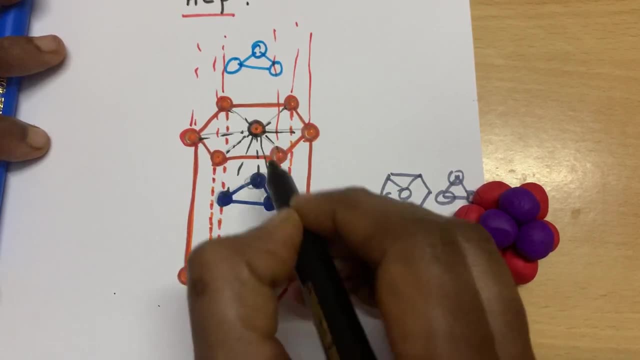 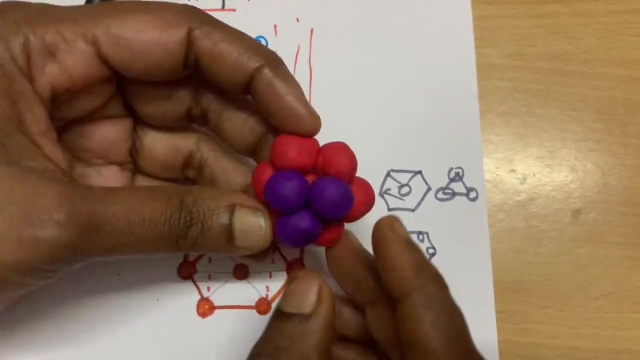 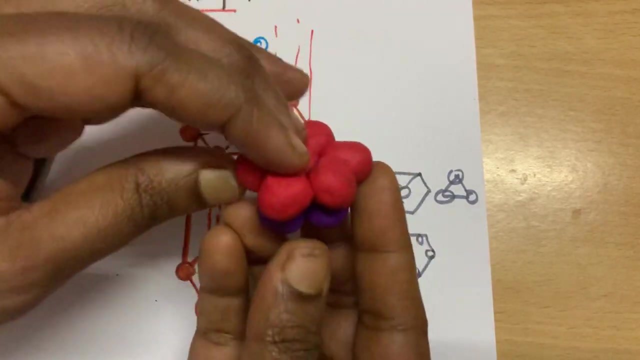 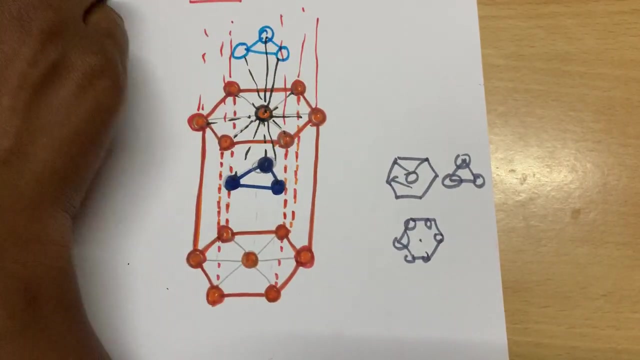 so it is coordinated. center atom is coordinated to this, these atoms and these three atoms, and above three atoms. So in this model you see center atom, center atom, one triangle, okay, one triangle below three atoms below and three atoms above three atoms above. so totally how many atoms? 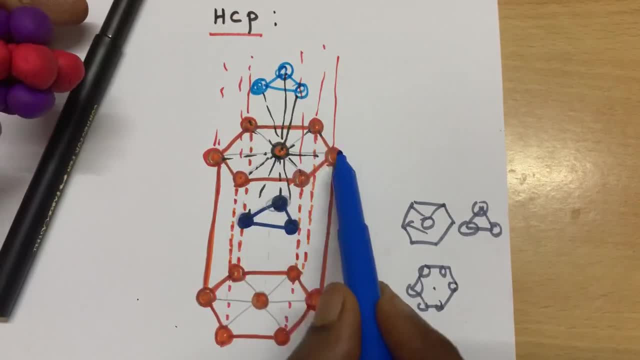 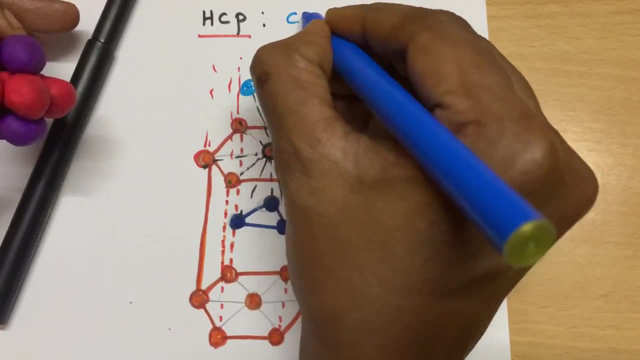 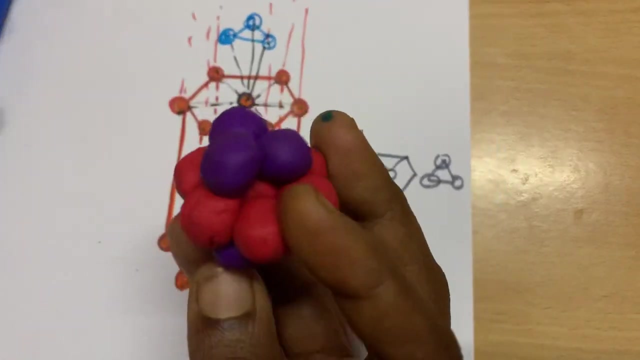 totally how many atoms: 1,, 2,, 3,, 4,, 5,, 6,, 7,, 8,, 9,, 10,, 11,, 12,. the coordination number for HCP is also 12, so I hope this was clear to you. so I tried my level best to make you. 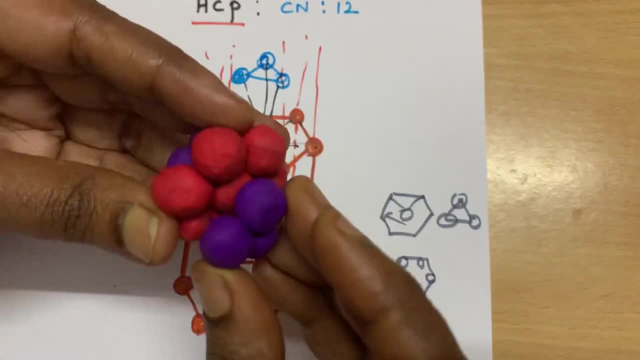 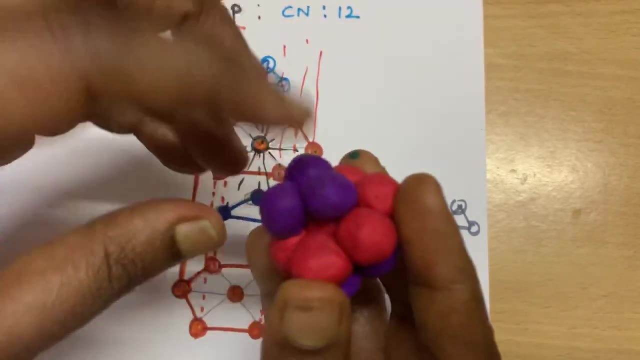 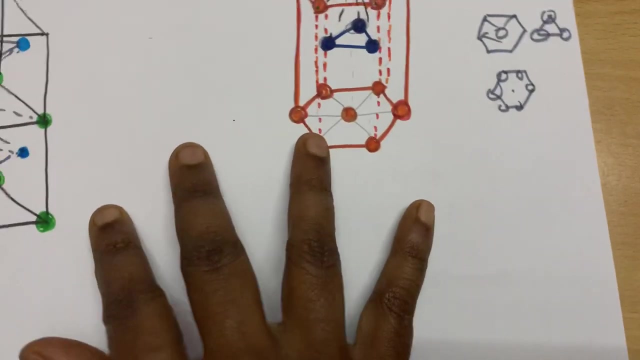 understand using the clay model. okay, so this is in touch. the center atom is touching the three atoms again. so downwards it is touching top layer also it is touching three atoms. okay, so totally it is 12,. so on concising the result for HCC: